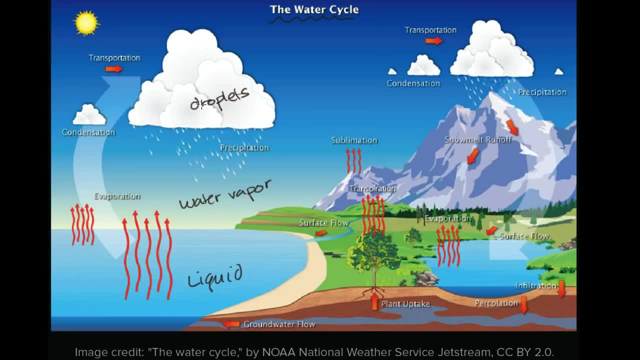 and they're condensing around these little microscopic dust particles To form these water droplets and if it's cold enough, they might also form small ice crystals, and that's what clouds are, And we see here they're talking about transportation. 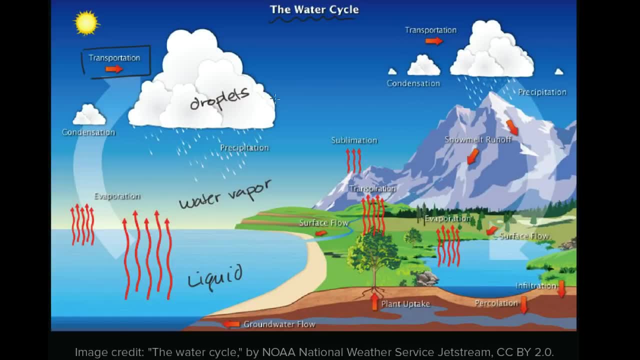 You can have these clouds, we. obviously, if you look outside and you see clouds, those clouds are moving with the wind, and so they could be moving all of those droplets with the overall wind, and when those droplets get heavy enough, they will precipitate. 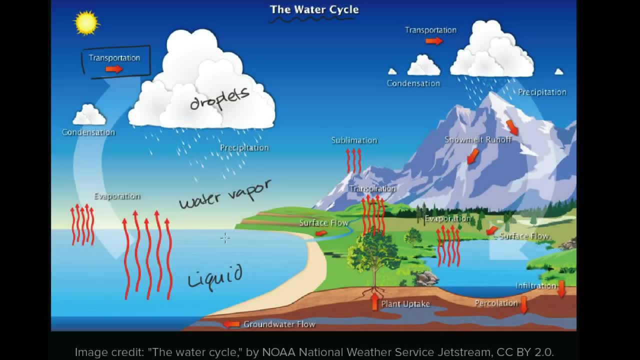 they will precipitate down Now. they could precipitate back into where we started. They could go back to the ocean there, or you could go onto a mountain here and, if the air is cold enough and if you have the right conditions, 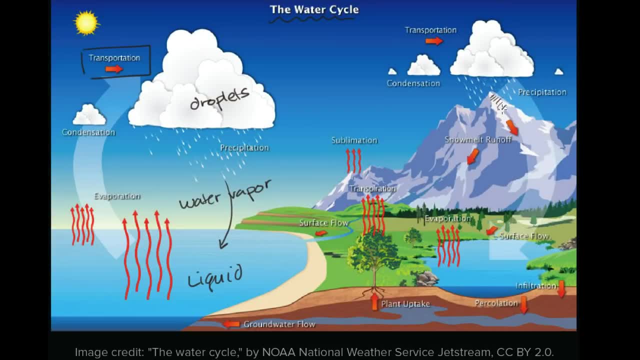 that precipitation might be snow- and it might stay snow right over there- or ice, But then eventually things might warm up or they might not warm up. but if they do warm up, well, then they would melt and then they would be. 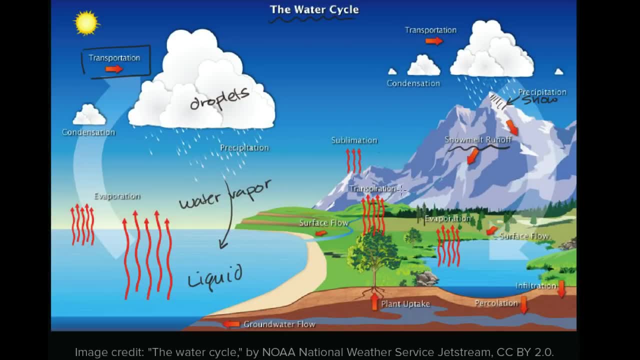 snow, melt, runoff, and that's what you're seeing there. If that rain is falling in this area- and, let's say, it's not cold enough for it to be snow, so we are talking about rain- well, most of that water is actually going to. 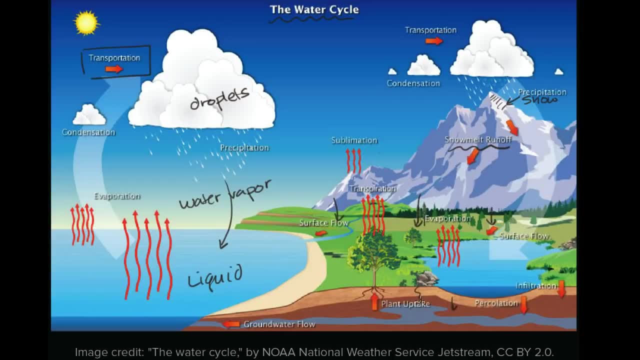 percolate down into the soil, So most of it goes down. we look around us and we see these rivers and lakes and we say, oh wow, there's a lot of water there. but it turns out there's actually a lot more water. 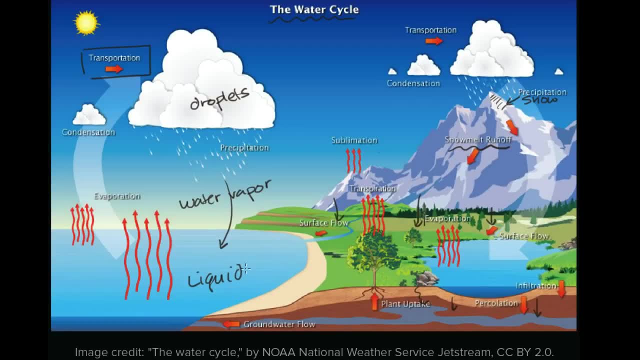 inside the ground and obviously in the ocean, and we'll talk about that in a little bit. And so you have these. you have all of this water that forms and these underground, these underground aquifers here, but some of it also ends up in these lakes. 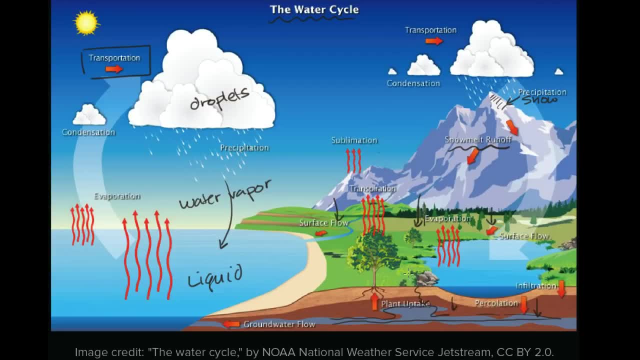 and these lakes are usually in a situation where the ground is either already saturated water or there's the right types of rocks so it can contain the water up here. And similarly, rivers are formed by runoff. it's snow melt, runoff can famously form rivers. 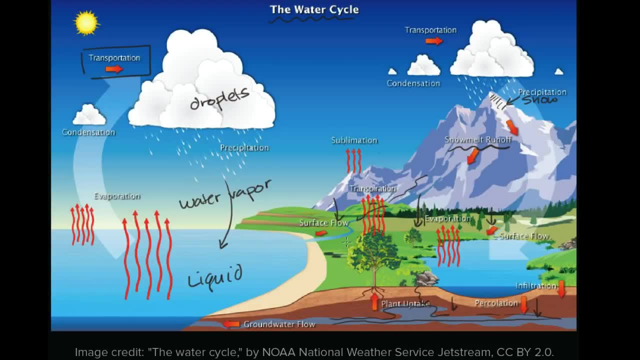 and, in general, if you see a creek or a river near your house, especially when it rains, it fills up. that's a good indication that the groundwater is already saturated and so things are running off into that river, And so that, in general, is the water cycle. 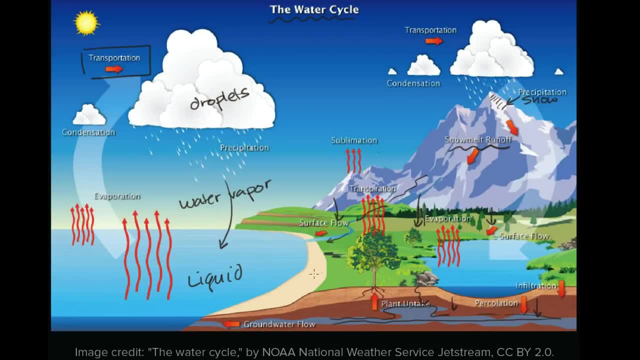 you have evaporation, it condenses into clouds, it eventually precipitates, and it keeps going round and round and round. Now, of course, there's other actors at play. you have things like plants. plants will take up water from the upper soil as far as the plant's roots go. 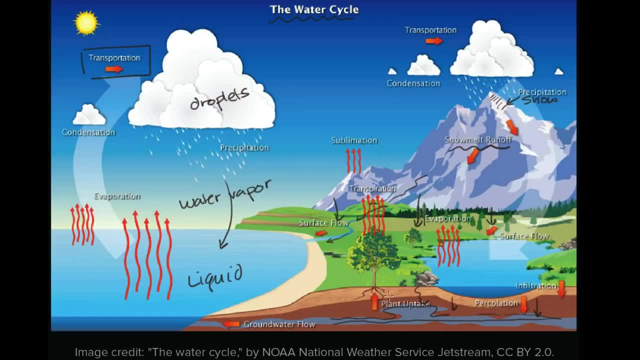 and it will use that water to transport nutrients down from the soil up into the leaves. it also uses that water as part of the photosynthesis process that we've studied in many videos, and a lot of that water gets transpired out. so, once again, this is transpiration. 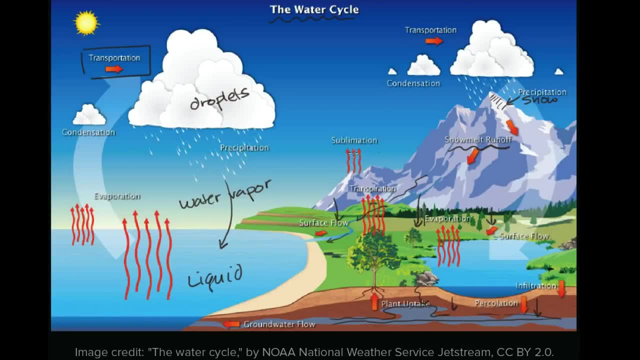 essentially evaporation out of the leaves of the water. Over here you see this word: sublimation, that's going straight from the solid form of water- ice- into the gas form of water or water vapor, And this will happen in situations. 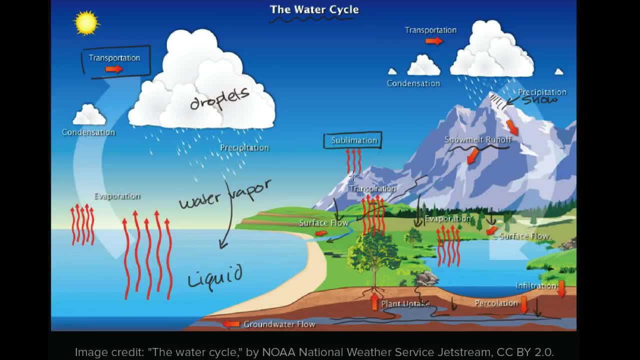 where it's cold and it's very, very, very, very, very dry, And you have, in general, low pressure. and so, right when, instead of going into the liquid state, right then the water molecules just start leaving. 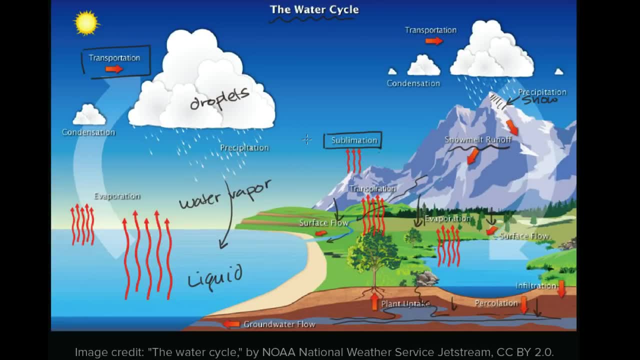 as water vapor Now, and of course I said we're part of it. well, how are we part of it? Well, we will drink some of this fresh water. our bodies are actually mostly water. the cells in our bodies are 70% water. 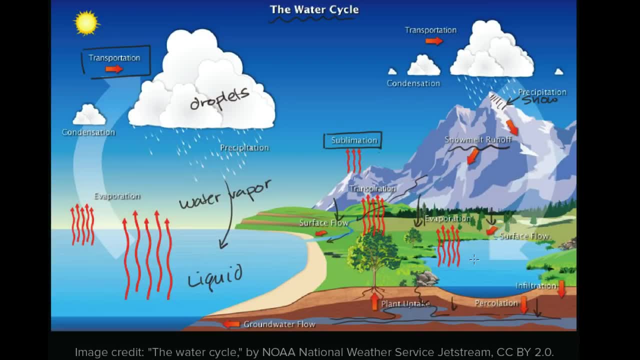 we. everything we study in biology, water is a key environment for all of these things to occur. and then we use that water and then we will. we will get that water out of our body and then it continues on is part of this water cycle. 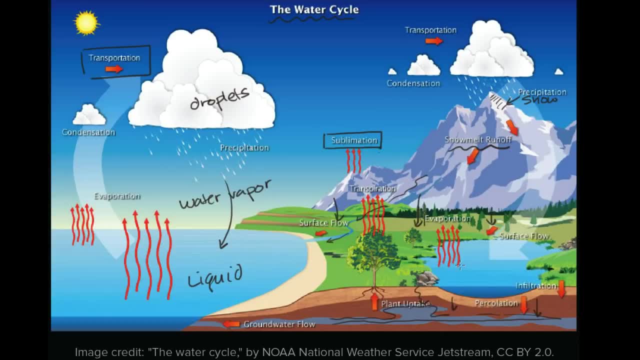 Now, one thing that I find really interesting as an organism that is dependent on fresh water. when people say fresh water, we're talking about water without salt, as opposed to salt water, so we really need this water, that's in the fresh water, in this lakes or in this river. 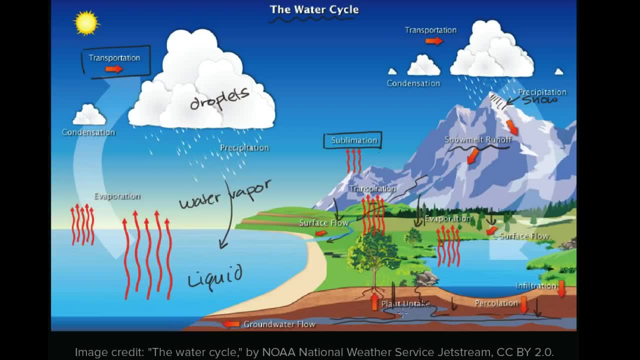 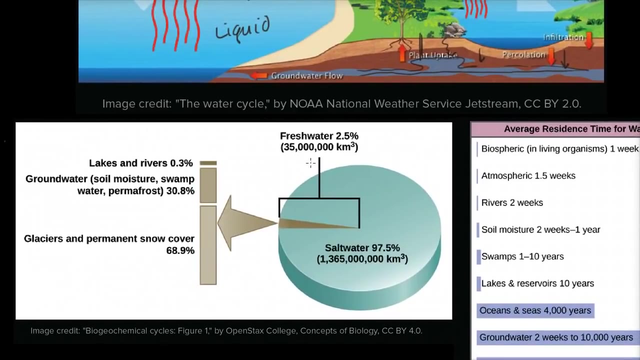 or we might dig wells so that we can get the water out of these aquifers. it actually turns out that very little of the overall water in the world is fresh water, and so let me show you this chart over here. I always knew that, but I didn't fully appreciate. 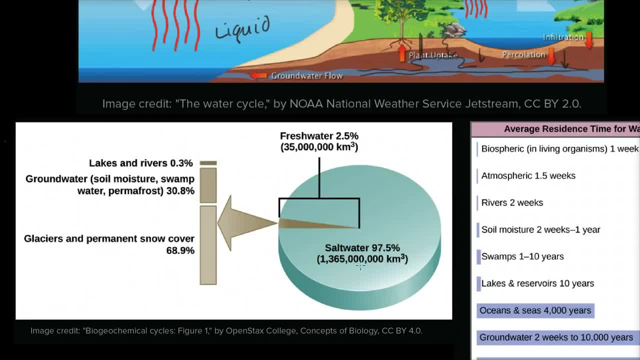 how little was fresh water. So of all the water on our planet, 97.5% is salt water, for the most part. in our oceans, only 2.5% is fresh water, and even of that, 2.5% fresh water. 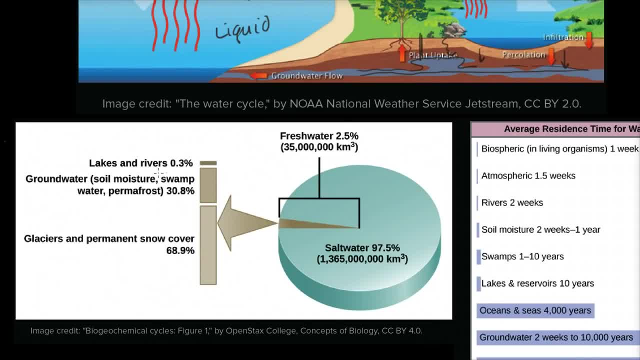 very little of it is what we traditionally associate with fresh water: the lakes and the rivers. When I think of fresh water, I mean let's say: oh, let me go to a lake or a river, that's stuff that we could potentially drink. 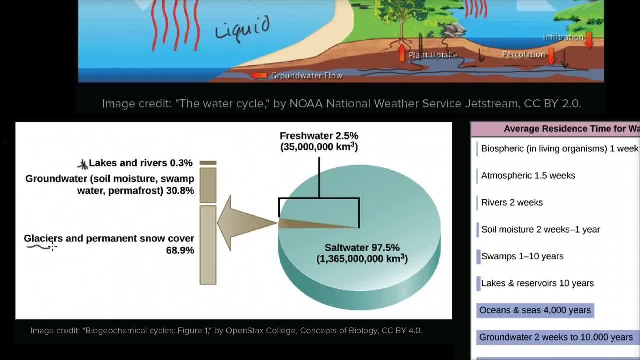 but most of it is actually in glaciers and permanent snow cover, So it's ice snow that is just not melting, and it makes you think about what would happen if this stuff were to melt And then you also have ground water. 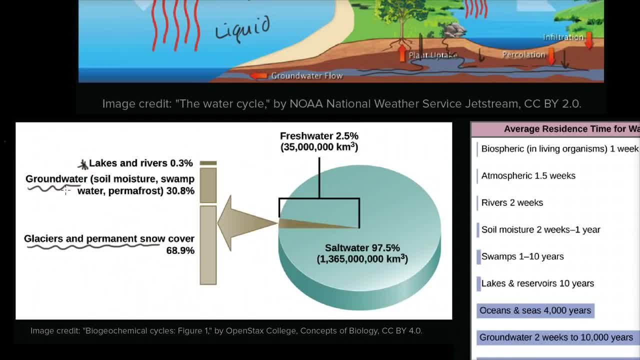 which we could have access to. that's why people drink dig wells, So we're talking about well ground water includes soil, moisture, swamp water and permafrost, but very little of the water is actually in lakes and rivers, which I personally find fascinating. 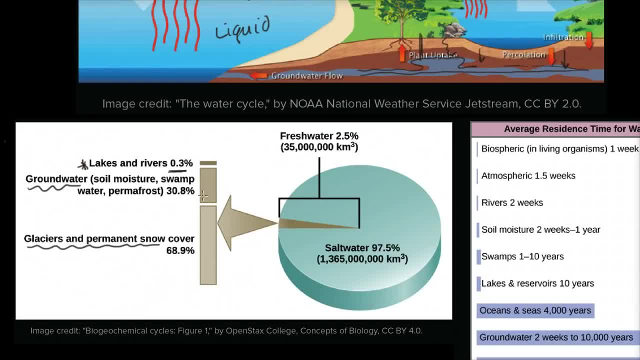 It wasn't obvious to me before. I, frankly, saw this chart. Now, another really interesting thing is how long, on average, water molecules might stay in different parts of this water cycle. So you know, going back here, you could imagine that a water molecule could stay for a very long time. 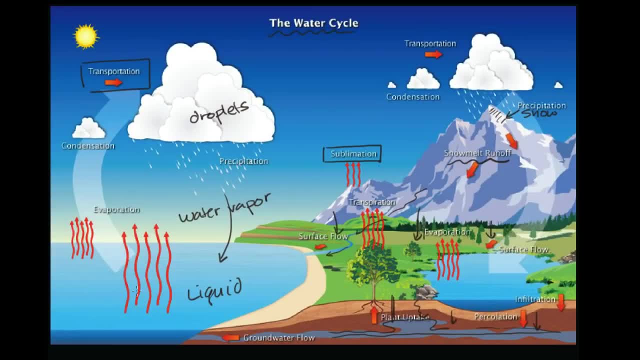 in the ocean especially, you know, moving around depending on ocean currents and temperature and all of that. but you could imagine it could stay in that liquid form in that ocean for a very long time and maybe it spends a shorter amount of time in a cloud. 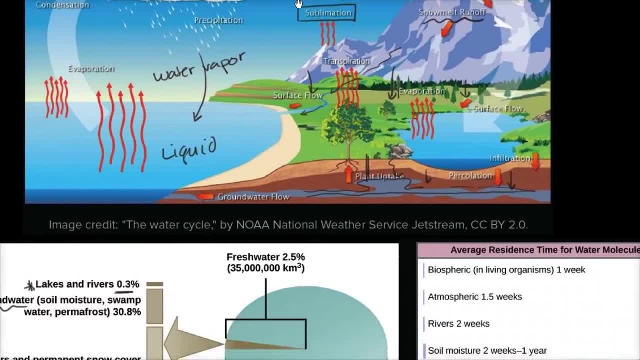 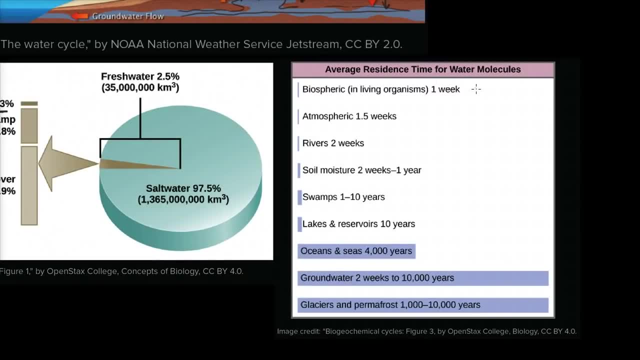 And people have actually studied this, which I find fascinating. I'd be curious to figure out how they actually got this data, But this is the average residence time for water molecules, and you can see here that water can stay in glaciers and permafrost for a very long time. 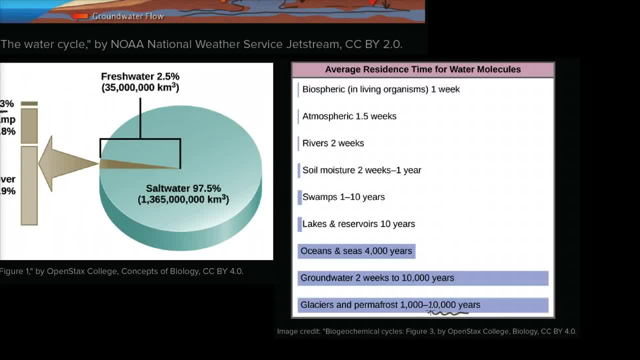 We're talking. it could be up to say 10,000 years, and these are all rough numbers. It could stay as groundwater anywhere from two weeks to 10,000 years, I guess, depending on how isolated that groundwater is.